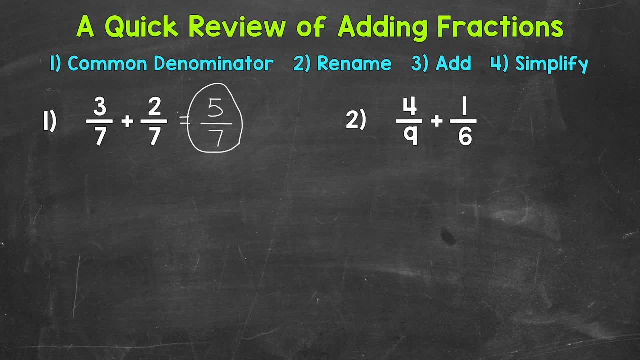 Now we're going to find a common denominator between 9 and 6.. By finding the least common denominator, So we're going to find the least common multiple between 9 and 6.. And that's going to be our least common denominator. 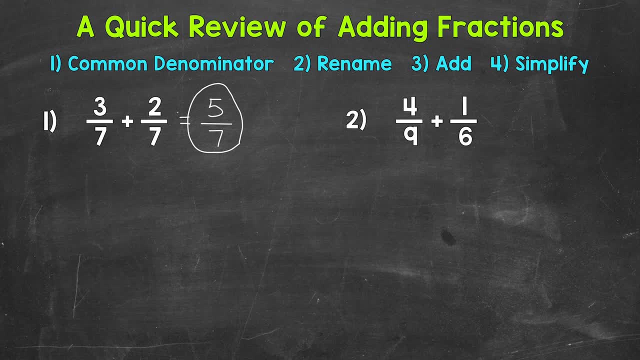 You may be able to think about what that least common multiple is, But as a review, let's write out some multiples of both 9 and 6 in order to find that least common multiple And again, that's going to be our least common denominator. 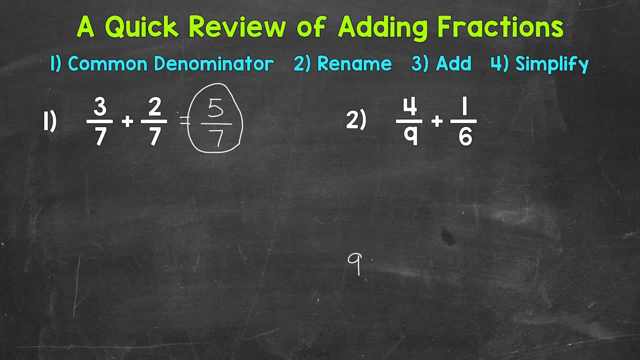 So I'm going to come to the bottom here. So 9 and 6. Now we can then add our denominator. Now we can list the multiples of 9 and 6 by just counting up by 9 and 6.. Multiples go on forever. 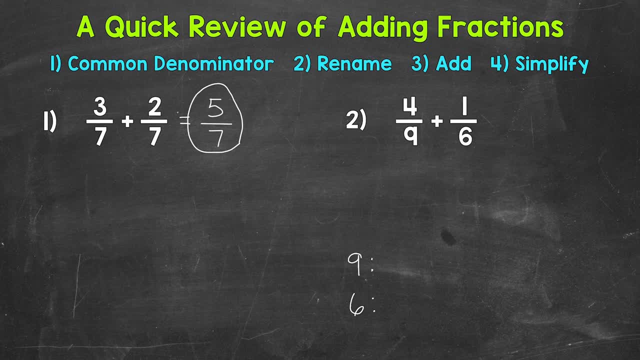 So what we can do, we can just start with 4 or 5. See if we have any in common, And then we can go from there. So let's write out 4 multiples of 9.. So 9,, 18,, 27,, 36.. 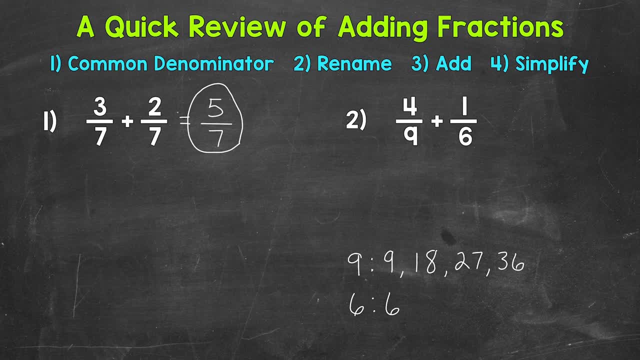 Let's write out 4 multiples of 6. And then see if we have any in common. So 6,, 12,, 18, 24.. It looks like we have 18 in common here, And that's going to be our least common multiple. 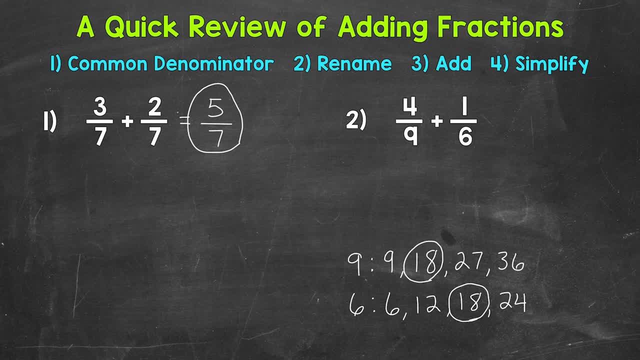 We're going to use that for our common denominator. So I'm going to rename these fractions underneath the original problem with that denominator of 18.. So when we rename we're going to use equivalent fractions. So we're not changing the value of the problem at all. 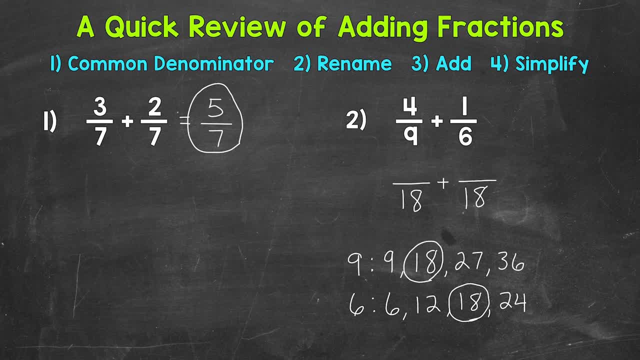 We need to think: how do we get 9 to equal 18?? Well, 9 times 2 is 18.. Whatever we do to the bottom, we have to do to the top in order to keep this equivalent. So 4 times 2 is 8.. 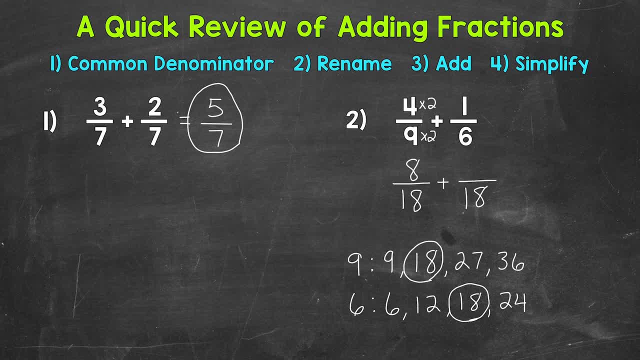 8 eighteenths is equivalent to 4 ninths, So that's going to be our least common multiple. So let's write out 4 multiples of 9.. Let's write out 4 multiples of 9.. So that's going to be our least common multiple. 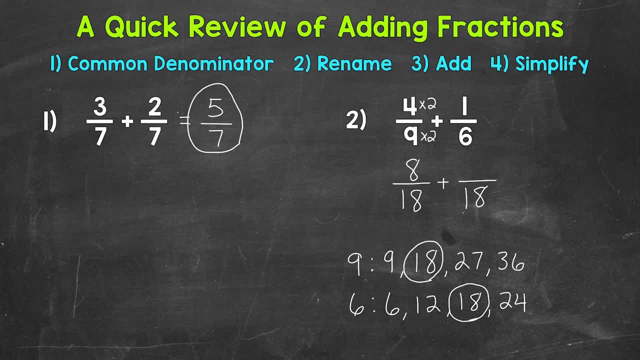 But we renamed that original fraction of 4 ninths with that common denominator of 18.. So again, we're not changing the value of the problem at all, We're just renaming with that common denominator. so we can add: Let's do 1 sixth. 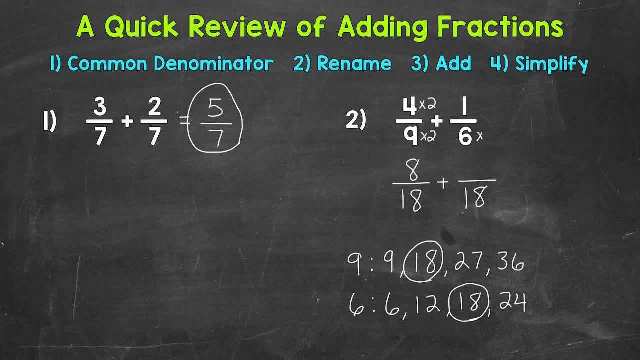 So how do we get 6 to equal 18?? 6 times 3 is 18.. So we need to do the same thing to the top in order to keep this equivalent. 1 times 3 is 3.. Now we have the fractions in our original problem, renamed with that common denominator of 18.. 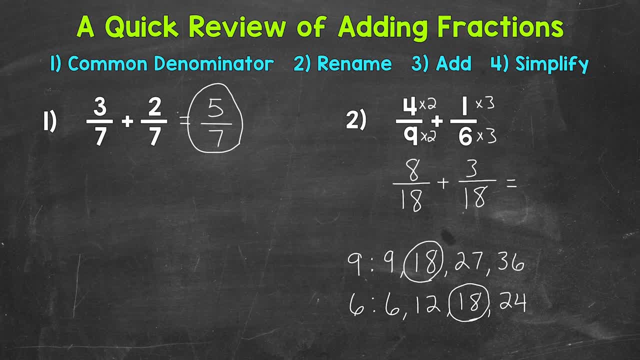 So we can add. Let's add our numerators: 8 plus 3 is 11.. And then we keep our denominator of 18 the same. Always. look to see if you can simplify 11 eighteenths. the only common factor between 11 and 18 is 1.. 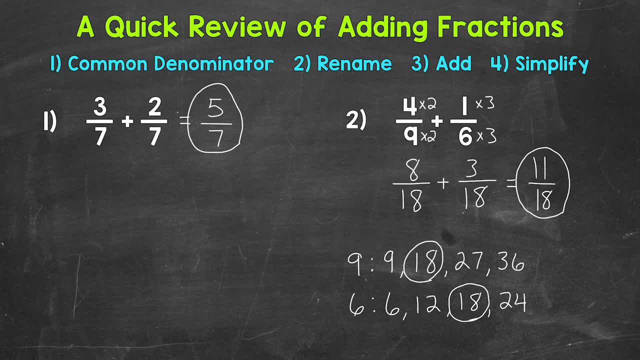 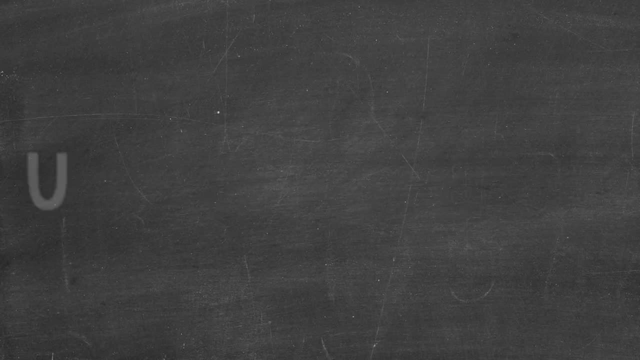 So we are in simplest form- And this is our final simplified answer- 11, eighteenths. So there you have it. There's a quick review of adding fractions. I hope that helped. Thanks so much for watching. Until next time, peace. 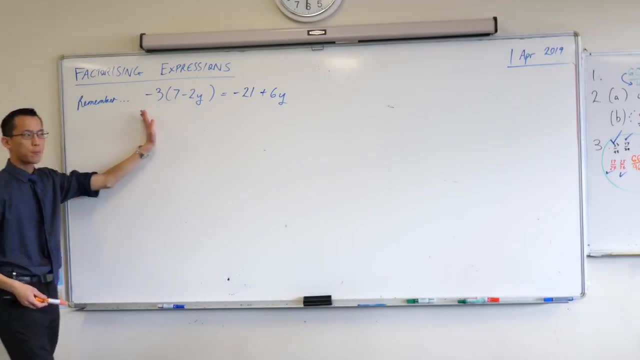 Underneath that heading. what I'd love you to do is: could you please jot down: this is something we did in question 2, it's 2B. it's just one part of it. Could you just jot down this equation again, please? 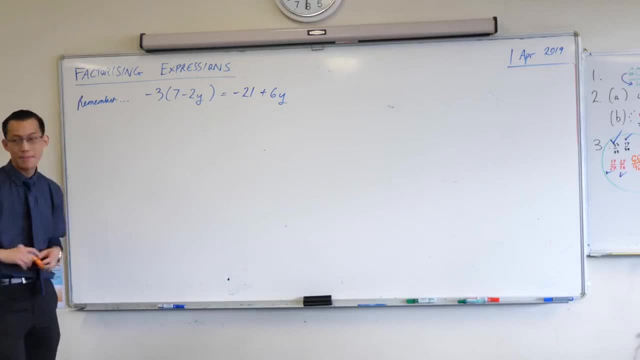 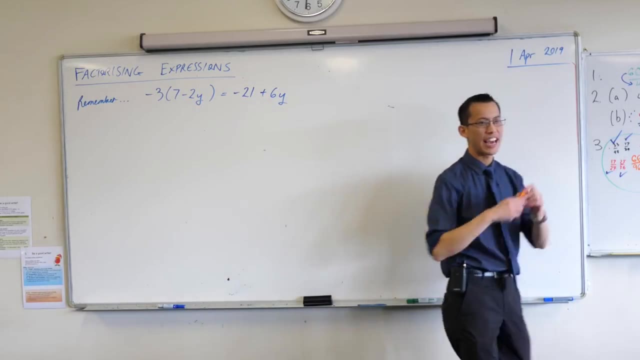 There's a very good chance you have working like it in your page already, but you might not, depending on what question you got up to Now. I did flag this before, but I just want to state it again so it's really clear, right. 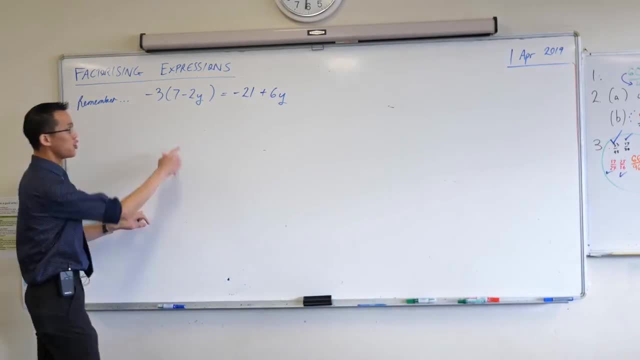 What you were doing during the quick questions when we started was: you went from here from the left-hand side to the right, and we gave that process a name. We called it start with an E- Expanding, Expanding. thank you very much. That's expanding.